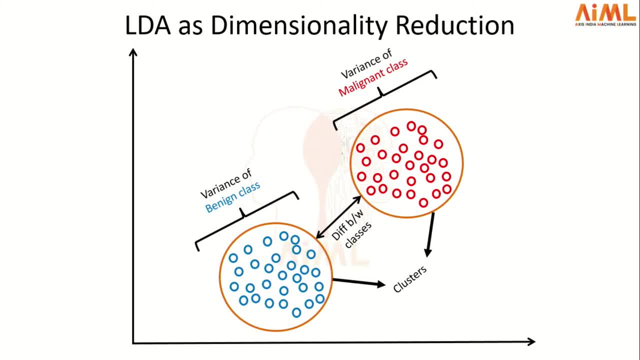 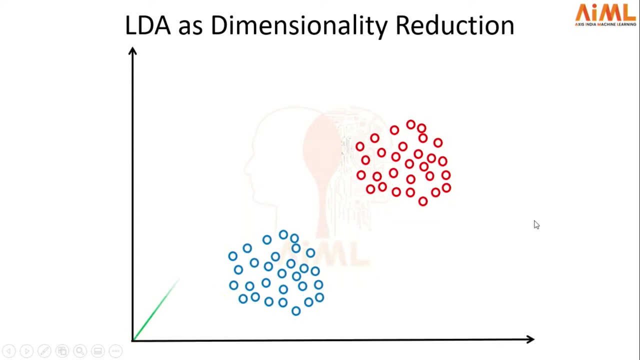 that two criteria should be satisfied. First criteria should be that the variance of the projected data point Should be reduced and the distance between the projected data of the individual clusters increases. So let us make the unit vector, and obviously here we are going to take some 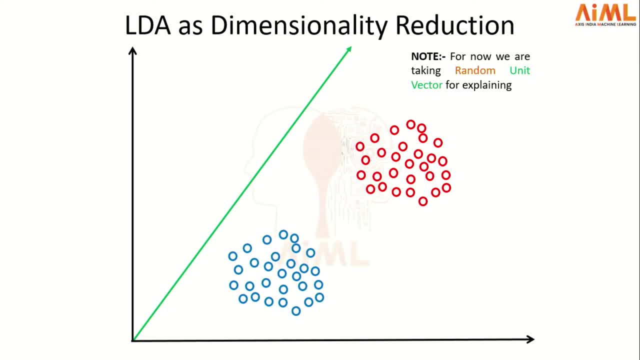 random unit vector just as an example to give you a visual effect of the concept Now when we start projecting the data points onto this unit vector. So these are the projected data points of the benign category and these are the projected data points of the malignant category, And here you can see that we have two clusters. 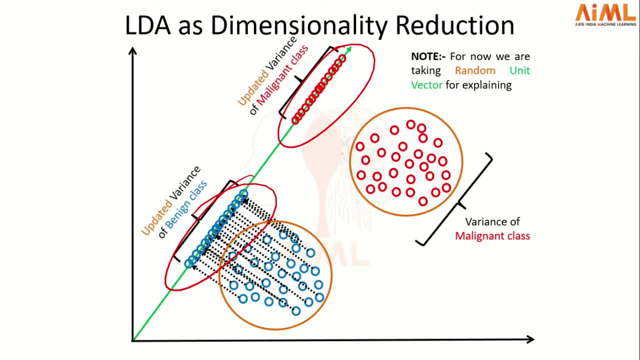 and you can clearly see that the updated variance of the projected data points is coming out to be little bit less in comparison to the variance of the data points which were not projected. So this width, or this width, is less than this width. In fact, the difference between 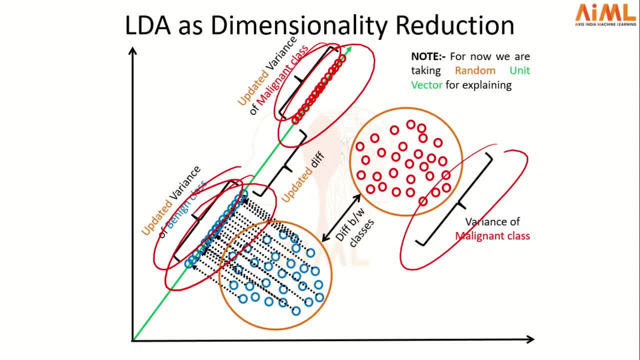 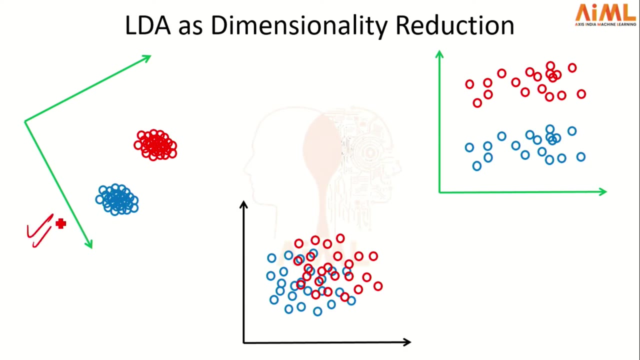 the projected data points is also increased. It means the two criteria are getting satisfied. So this difference is less, whereas this difference is more. So now let us try to visualize that: how LDA projects: different kind of data in different scenarios. So we have here three scenarios. So let us see the first scenario, that where LDA projects. 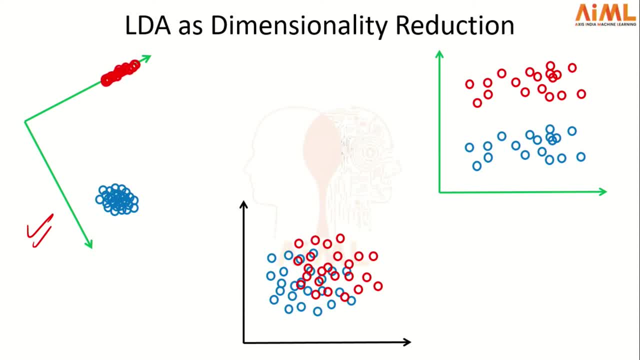 this data. So LDA will definitely choose the above unit vector to project the data because the two criteria are getting satisfied. In the second scenario you can clearly see that where the LDA is going to project the data points, it will project to the side because 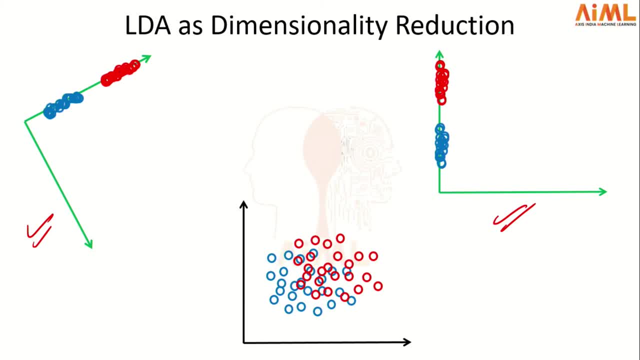 obviously the two criteria are getting satisfied, But the third case is pretty interesting. So what happens if LDA projects the data points to a single unit vector and the data is not being able to be classified into one unit vector? like basically the same argument. 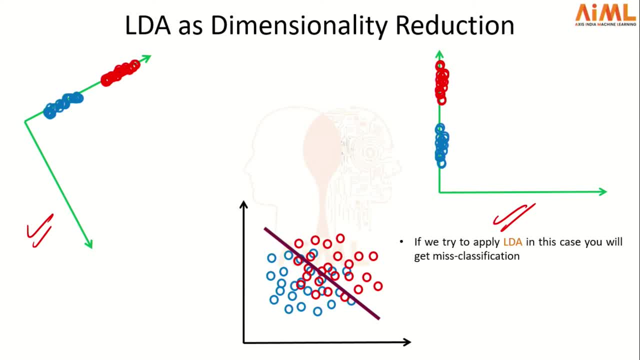 what happens. The data points are not being classified as it should be, and we would be missing this case, Because in this case, if we try to project the data points onto a unit vector, we get quite a good amount of misclassification. Okay, so in this case, LDA is not a good option.